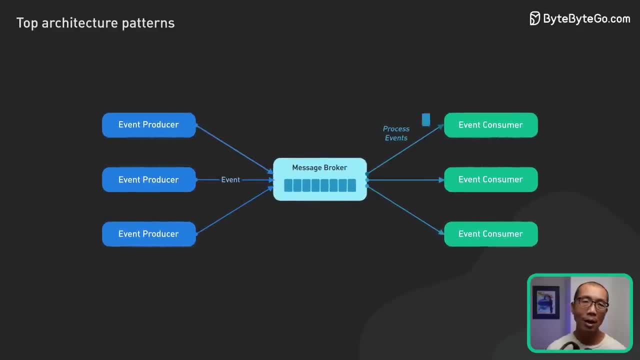 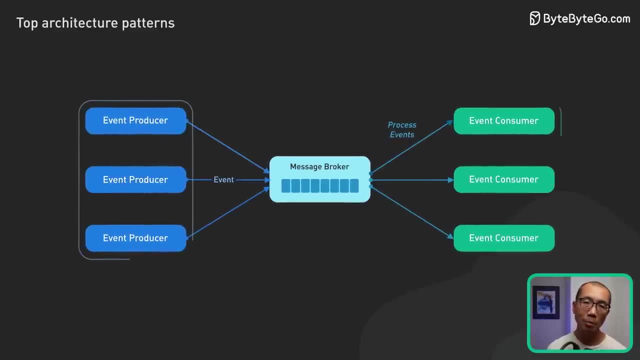 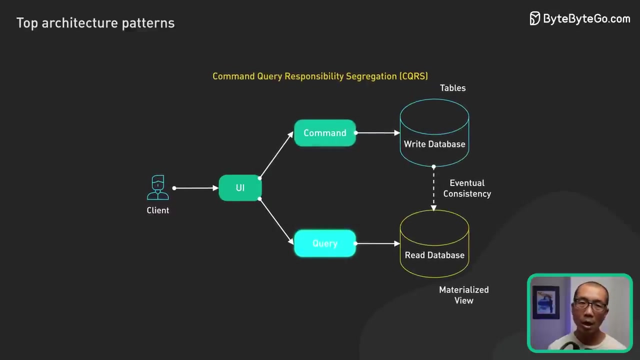 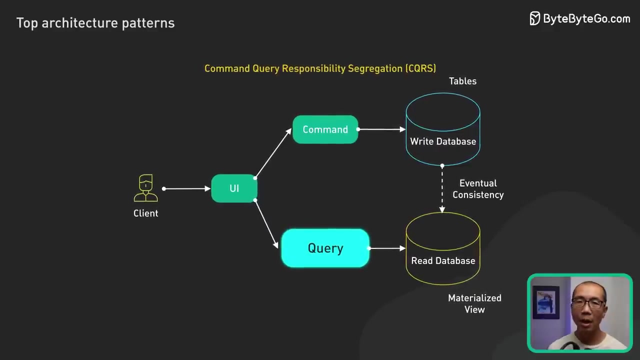 Components broadcast events when something notable happens and other components subscribe to specific events they are interested in. This allows for highly decoupled architectures. One prominent example in this domain is CQRS. With CQRS, the data write operations commands are separated from read operations. queries and changes are often communicated through. 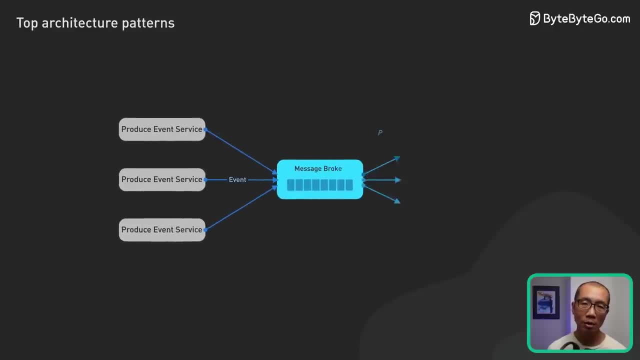 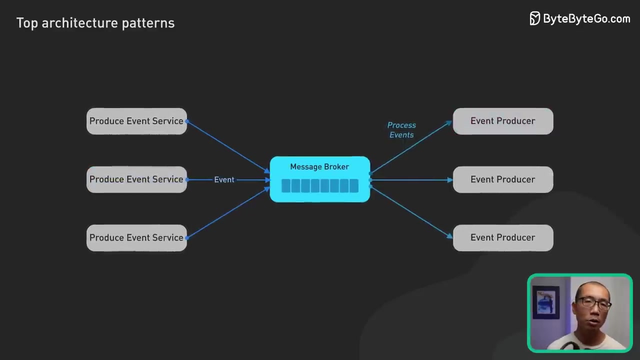 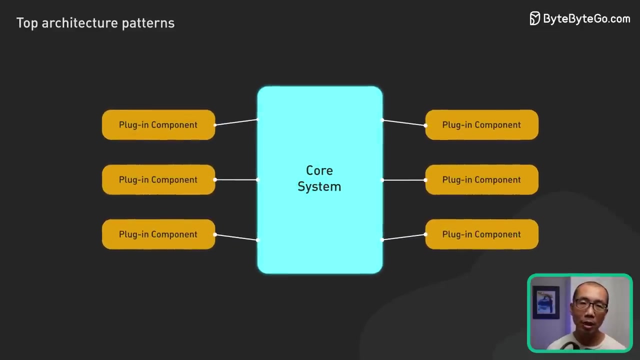 events. This makes the system inherently event-driven. The Pub-Sub model, where components publish and subscribe to events, is commonly used in such architectures. Here, components don't call each other directly, they merely react to published events. Moving on to microkernel architecture, This pattern emphasizes separating core system. 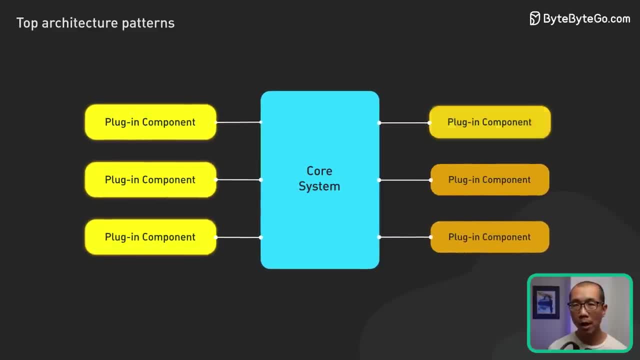 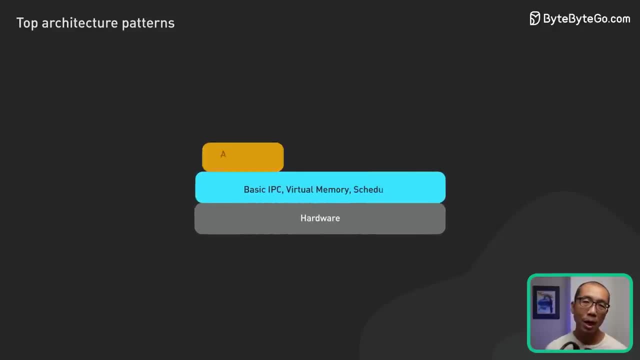 functionalities into a small microkernel and extend the functionality into add-ons or plug-ins In operating systems. for example, a microkernel might oversee vital tasks like inter-process communication, while offloading other system functions to external components. An application example is the Eclipse IDE. Its core runtime handles the plug-in architecture. 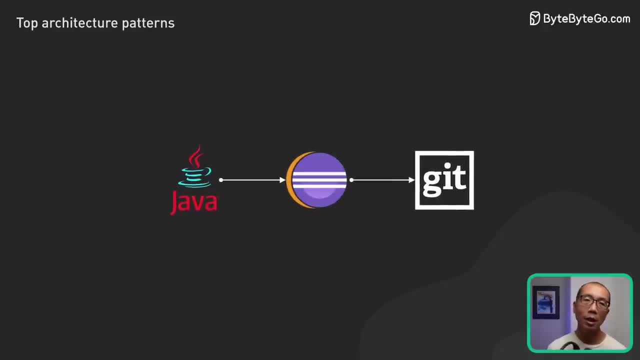 and features from Java tools to Git integration are delivered as plug-ins. This design prioritizes extensibility, ease of maintenance and fault isolation. Whether it is an OS component or an Eclipse plug-in that encounters an issue, the core system remains stable and unaffected. 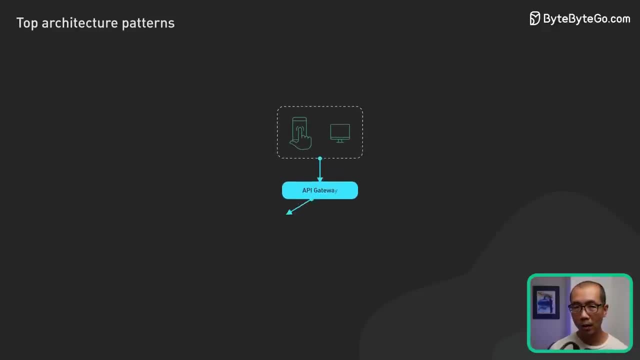 Then we have microservices. This decomposes an application into a collection of small, loosey-coupled services. Each service implements specific business capabilities, contains its own data model and communicates via APIs. Netflix, for instance, uses microservices to handle everything from movie recommendations. 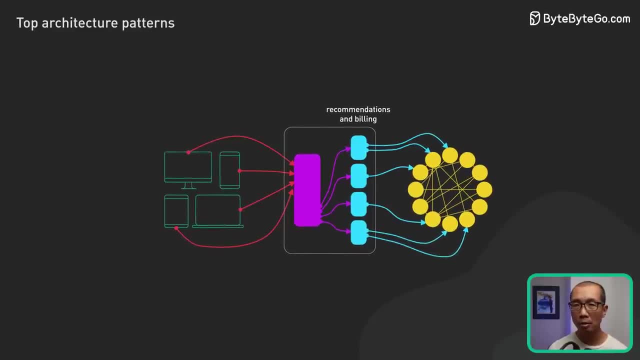 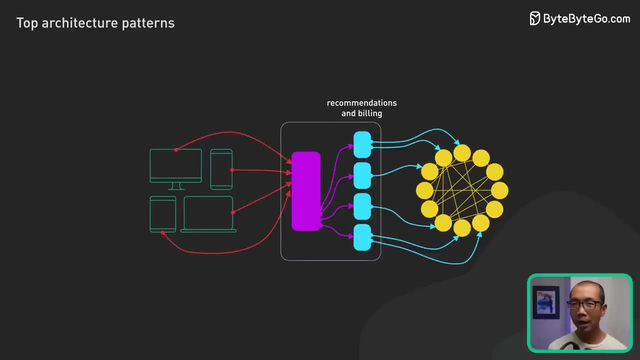 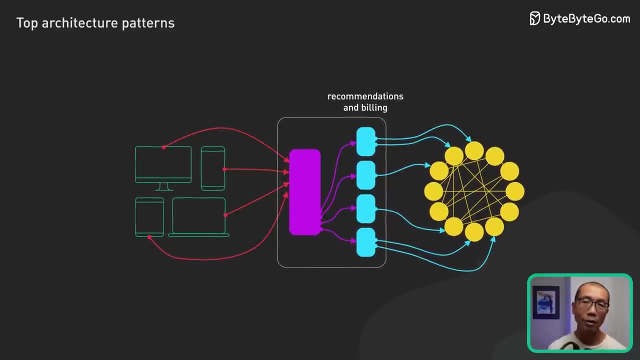 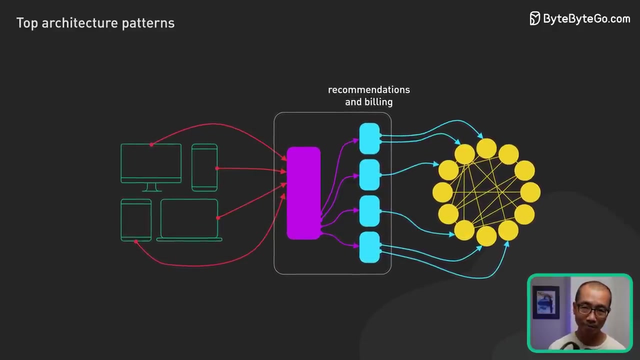 to billing. This architecture promotes modularization of functionality, so services can be developed and scale independently. It increases agility and allows companies like Netflix to rapidly innovate. The trade-off, however, is the added complexity in managing inter-service communication and maintaining data consistency. Last but